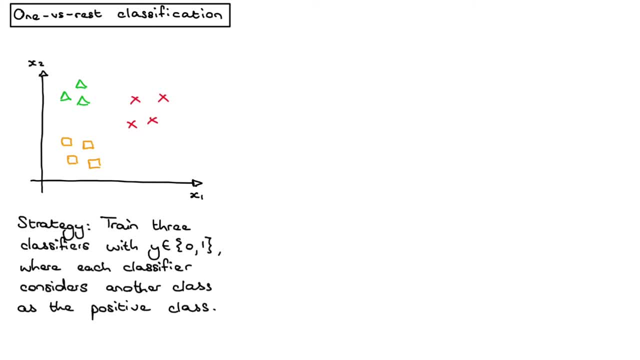 classification, but can do multi-class classification, telling us whether a new input point- let's say one here- belongs to triangles, crosses or squares. So the strategy is that we're going to train three classifiers. each of them is going to be a binary classifier and then we're going to see how we can combine them. 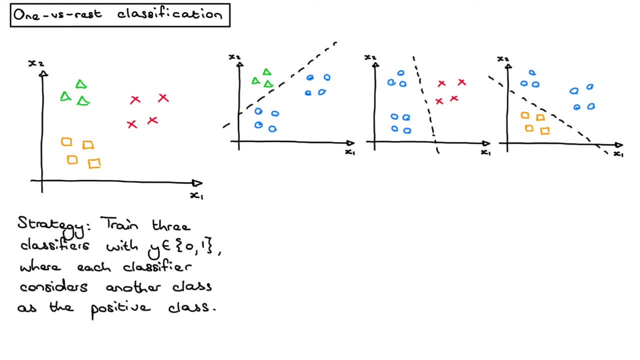 So step one is to train three different classifiers. The one is just a classifier for predicting whether something is a triangle or not. The second one is just one for training a predicting whether something is a cross or not. And the third one is something to just predict whether. 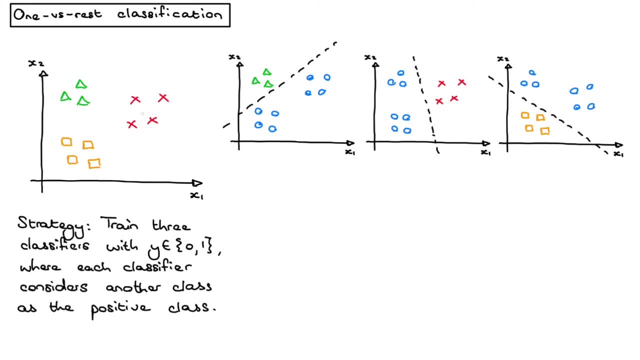 something is a square, square or not. All three of them are trained on the same training data, but obviously the labels for whether something is positive or negative are different in these three cases. So you build this kind of bank of classifiers, one for each of the classes that you're interested in. 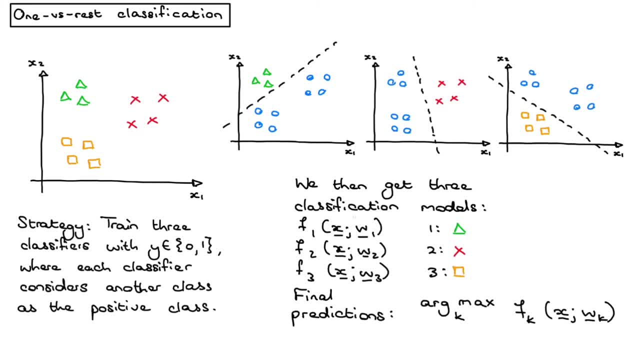 And then what you do is, at test time you're given a new input x, your new input x, and you don't know what it is. but what you do is you pass it through the first model, the second model and the third model and you get an output score. You can think of it as a probability for each of. 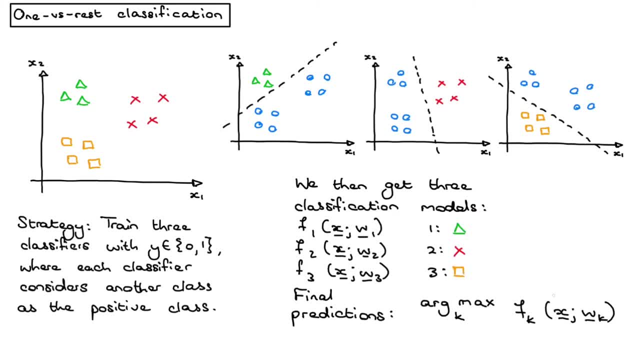 the three classes, for the triangle, the cross and the square class, And then what you do is you simply predict the class for which the score from that model is highest. So, if this is our first model- F1,, if this is our second model- F2, and this is our third model, F3,, 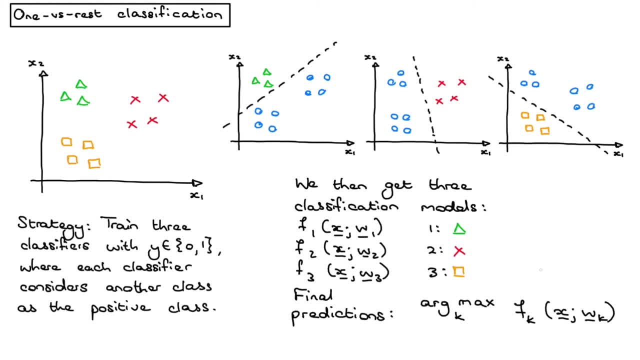 then what you're going to do is the final output of your model is simply going to be the model K that gave us the highest score for this input. Each of the three models will have its own weight vector, so we will have a W1,, a W2, and a W3, and we combine all of them together. 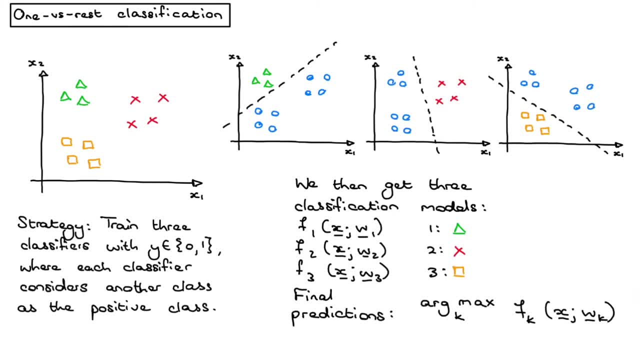 into a single prediction like this Super simple approach turns out to work well in many cases, and you don't have to do this just with logistic regression. You can, in fact, take binary machine learning model and convert that into a multi-class classification model by using.